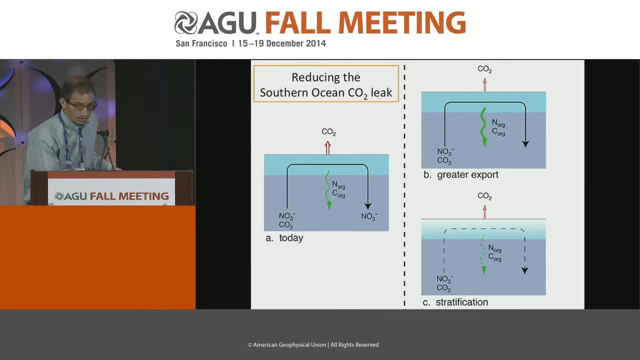 And because of limitations on phytoplankton growth in this environment, especially limitation by iron, phytoplankton are unable to completely reconsume the nutrients and excess CO2 that are brought to the surface As a result. some of those excess nutrients, a lot of them- return back into the interior. 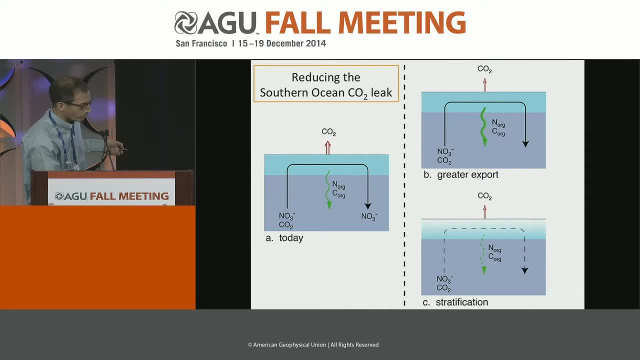 They're unused- I'm describing the nutrients here simply in terms of nitrate and CO2- is evaded to the atmosphere. So this is the leak. So since the discovery of glacial and glacial CO2- change of lower CO2 levels during ice ages- it's been recognized that if we could stem this leak during ice ages, we'd have a potential explanation for the lower ice age atmospheric CO2.. 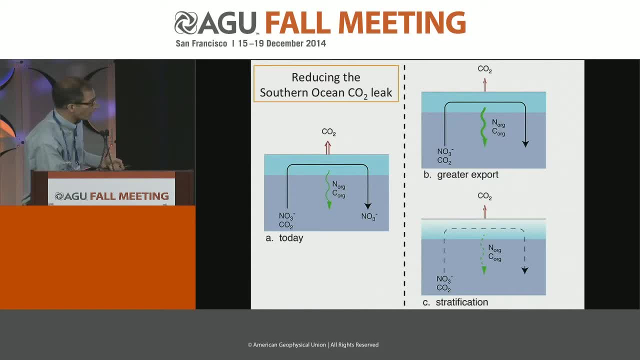 And in this context, there are two scenarios- end-member scenarios- that one can imagine. One is simply that Southern Ocean biology organic matter production in the surface and export to the interior increased and thus consumed a greater fraction of the nutrients and CO2 that are brought up, stemming this CO2 release to the atmosphere. 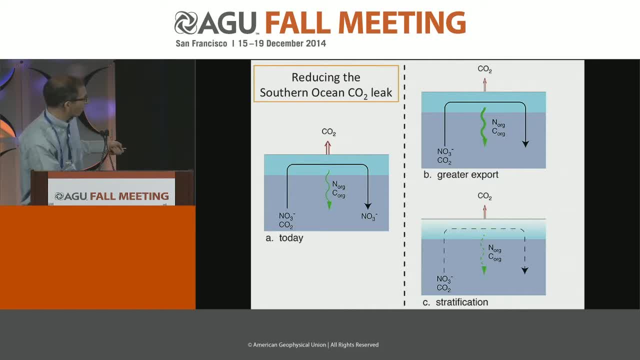 The end-member alternative, which I'll be describing as stratification through the talk, although that's not a terrific term- involves a reduction in the overturning rate through the Southern Ocean. This reduces the CO2 leakage by two ways. First of all, it decreases this overturning relative to other deep water formation processes in the global ocean, which, in effect, lowers this CO2 leakage. 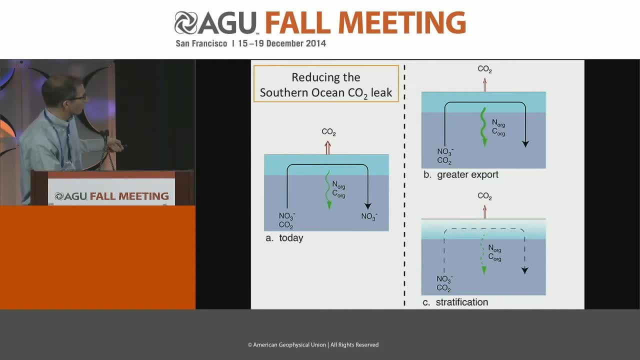 And, in addition, even if phytoplankton growth is constant or even decreases during the last ice age and during ice ages, this production would have been able to consume a larger fraction of the nutrients and CO2 brought up from below. So again, stemming. 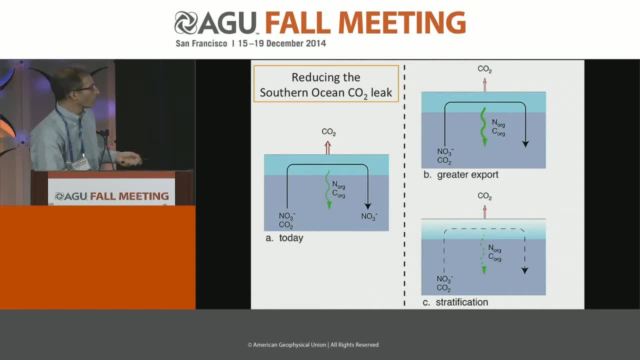 This CO2 leak. Now, the first type of work that people did to try to understand what the Southern Ocean did biogeochemically during the last ice age involved reconstructing export production, the flux of organic matter to the seabed- And in this work, what they observed was an increase in productivity in the ice age sub-Antarctic, but a decrease in the ice age Antarctic. 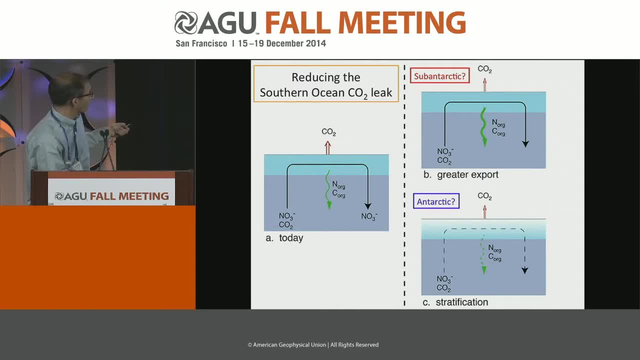 So for the sub-Antarctic, there was some greater. There was some greater excitement in the sense that it would be quite easy to imagine that this scenario would apply to the sub-Antarctic productivity increase. It was also recognized that there was an increased dust flux to the ocean during ice ages, which was what drove John Martin to propose the iron fertilization hypothesis to explain lower CO2.. 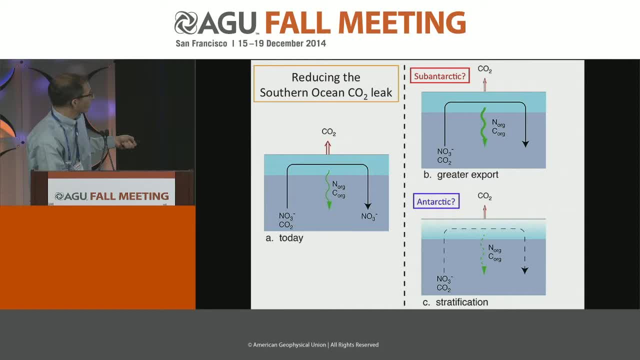 And so this has been something that people have been thinking about for a long time. The Antarctic was, at first, I think, sort of depressing this observation of lower export production In terms of the entire Southern Ocean playing a major role in glacial and glacial CO2 change. 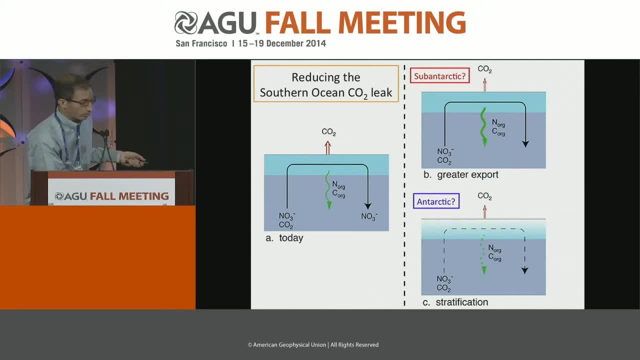 Here, export production was observed to decrease during glacials. So if the Antarctic, if you were going to be optimistic and argue that the entire Southern Ocean was working to reduce CO2 during ice ages, including the Antarctic, the Antarctic would have to be operating by this type of scenario, the stratification scenario. 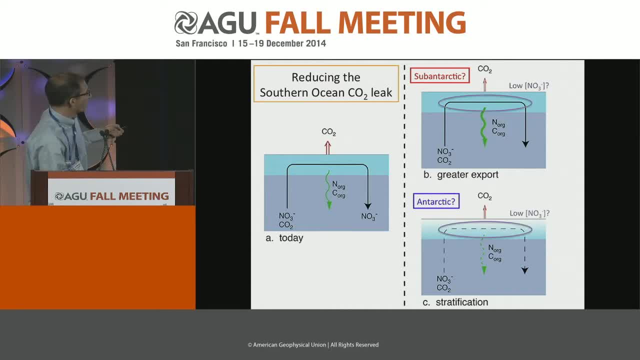 Now, one prediction that Both of these scenarios would make is that the degree of nitrate consumption would become more complete in surface waters. the nitrate concentration would fall in surface waters and we should be able to detect this as an increase in the N15 to N14 ratio of the organic matter that's produced in surface waters and exported to depth- an increase in the N15 to N14 ratio, and this is the same as an increase in the delta N15.. 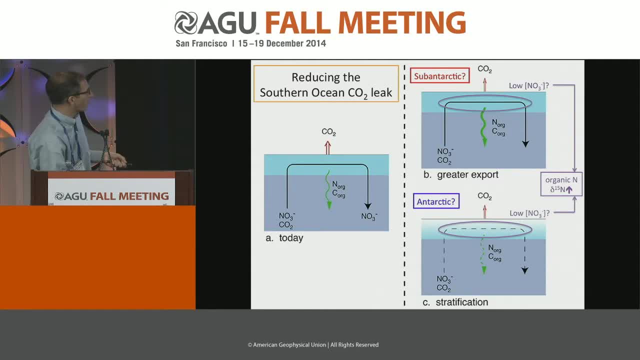 The first work that was done on this used bulk sedimentary nitrogen, but bulk sedimentary nitrogen is vulnerable To diagenesis and to contamination, and so today I'm going to be showing you data from organic matter bound within microfossils and diatoms in the Antarctic and foraminifera in the sub-Antarctic. 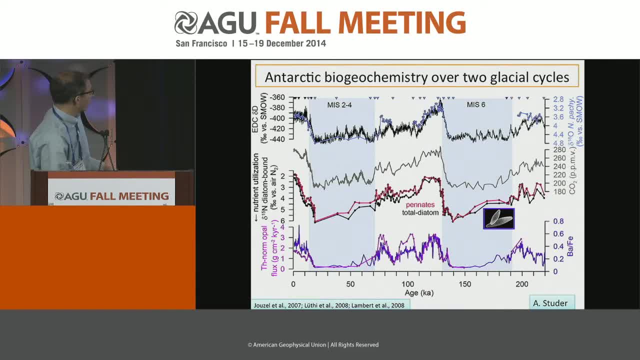 So now we're going to look at some data from the Antarctic. This is a core from the Pacific Antarctic sector. The data from the core is down below. There are a couple of curves from the ice cores up on top, So here we have atmospheric CO2 from the ice cores. 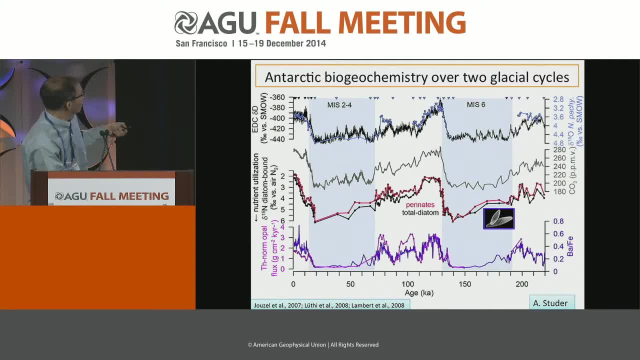 And a reconstruction of air temperature based on deuterium from the ice cores as well, And these on this time scale, we've got the ice ages here, the interglacials here, So the blue is the deeper part of the ice ages. 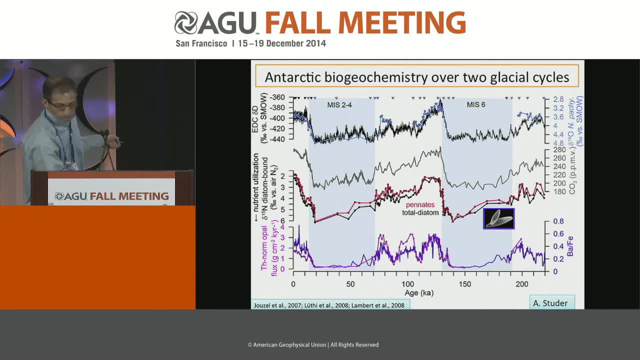 The data from the from the. is it counting down Good? The data from the sediment core is shown down below. So on the bottom here we have two proxies for the reconstruction of export production and, just as I said, they indicate that there is lower export production in the last ice age and in previous ice ages. 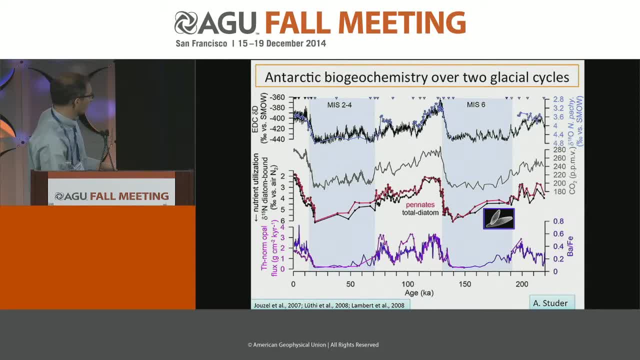 relative to the interglacials, as has been observed before Now. above that are the diatom bound nitrogen isotope data, and there are two records here, Both of which make me thirsty. There are two records here. The distinction is not particularly important for today. 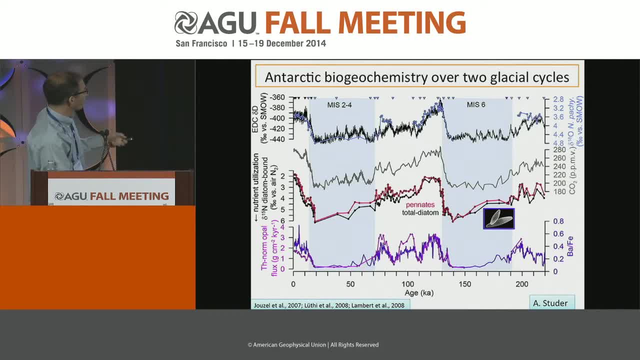 but they are actually independent records And so they give you some sense of our ability to ability of our measurements to reconstruct the relevant patterns. What these records show is higher, so I should say N15,, N14, or delta. N15 is plotted increasing downward here. 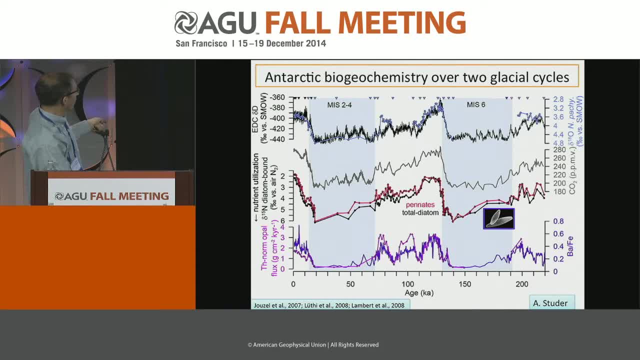 So increased nutrient consumption would be downward on this plot. higher surface nitrate concentrations would be upward. So what we're seeing for the ice ages is more complete nitrate consumption, Lower surface nitrate concentrations during the ice ages. And yet this is when these are times when export production, biological productivity, appears to be lower. 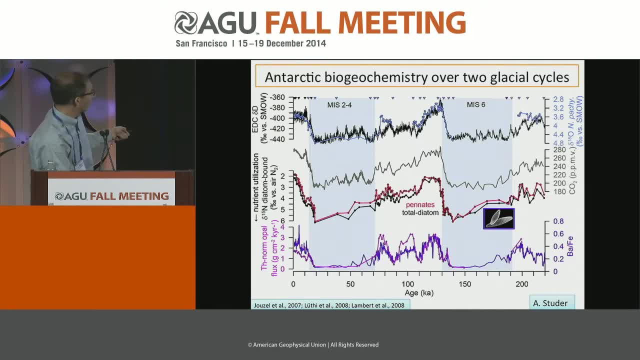 So the only way for both of these things to be true- higher degree of nitrate consumption but lower export production- is that there was a reduction of nitrate supply from below, ie something like that stratification scenario I proposed to you. 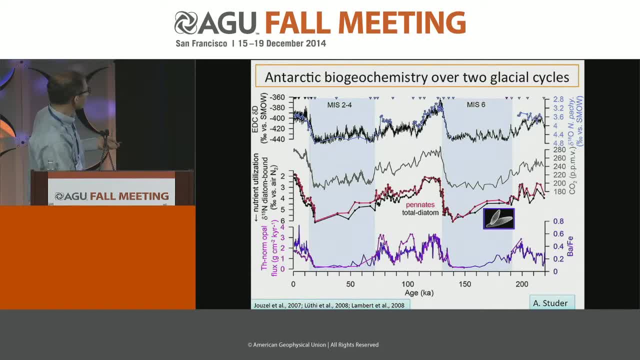 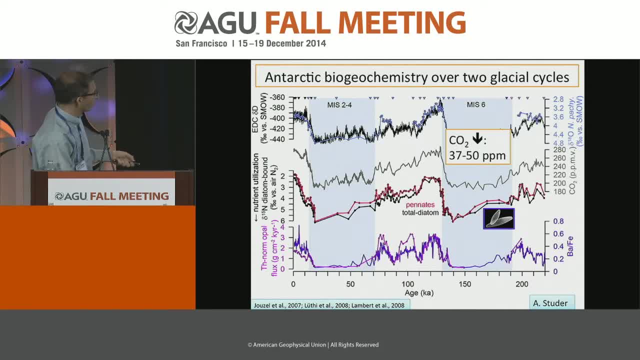 on box model simulations would suggest that the CO2 drawdown one would get would be something like 35 to to 50 pm, Lower numbers tending to apply when you're imagining this occurring in in the context of North Atlantic deep water circulation such as we have today. 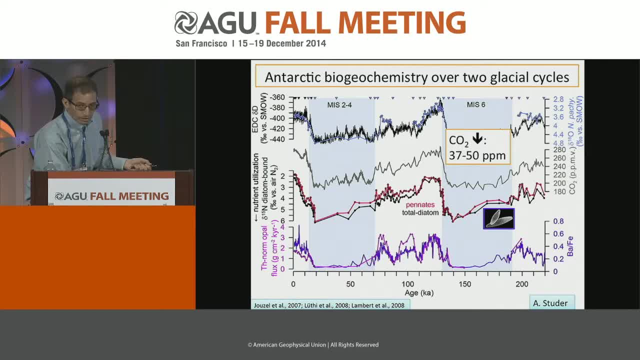 higher values tending to apply if you imagine glacial North Atlantic intermediate water forming in in the ice ages. One other interesting thing I want to point out here is that the diatom bound delta, delta N15, rises. 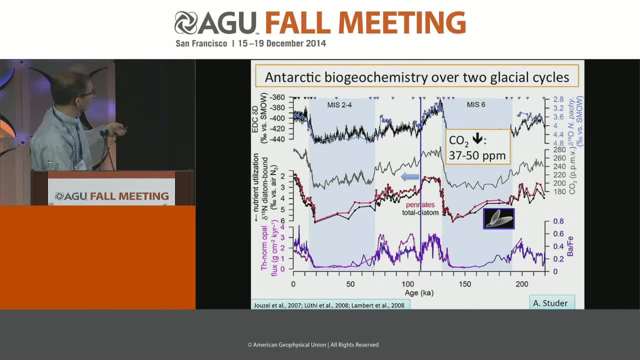 begin quite early in the glacial progression for the last glacial cycle, With the end of the previous interglacial. here we start to see the first increase in diatom bound delta N15. And so this 35 to 50 ppm CO2 decline can be applied. 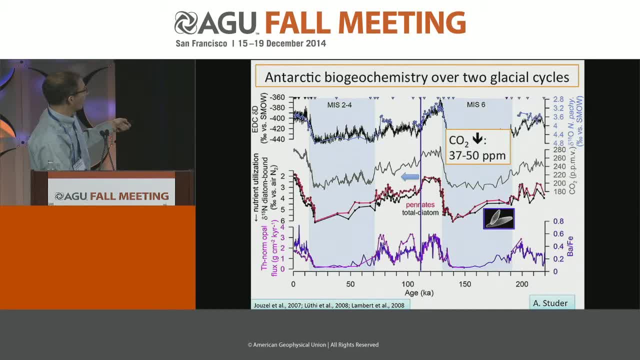 to this record starting from that time forward, and may help to explain, for example, the CO2 decline we see over this period, as well as some of the CO2 decline that occurs later on. Okay, so now let's move on to the sub-Antarctic. 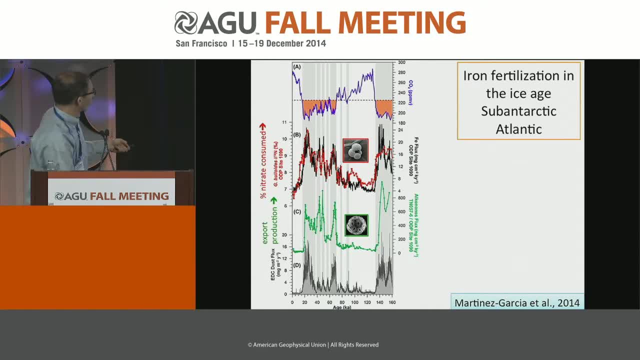 This is a quote from the sub-Antarctic Atlantic, the work chiefly of Alfredo Martinez-Garcia. So the data here we have on the x-axis age, again back to 160,000 years ago. Again we have some data from the ice cores plotted as well. so this is the CO2 record. 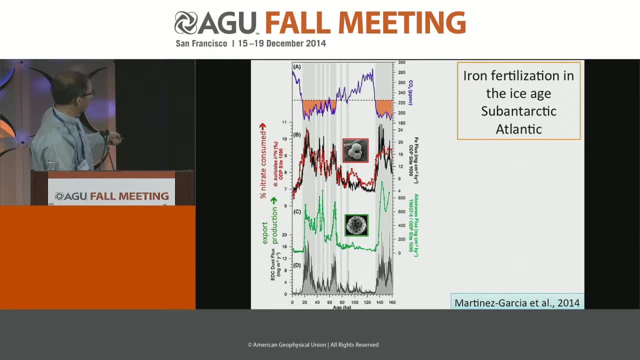 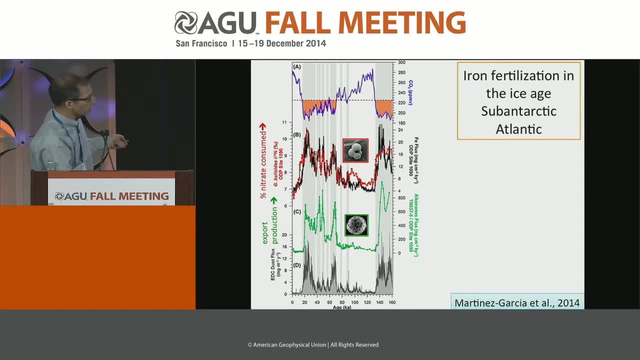 The idea would be would fertilize the southern ocean with iron and increase productivity. Quite remarkably, at this sediment core the iron fluxes follow the dust record seen in Antarctica quite well. So that's shown in the black curve up here that's covered by the red stuff that I'll. 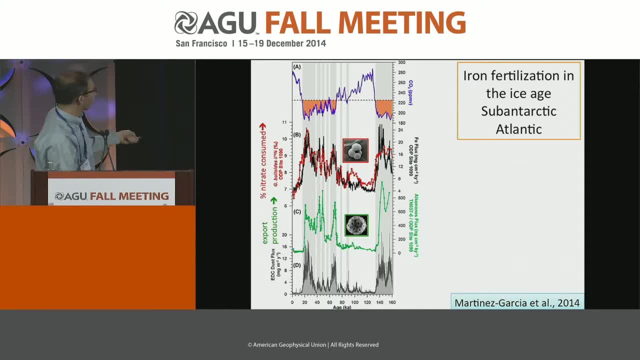 get to in a second. And so these dust fluxes that applied in Antarctica also, these dust flux changes that applied in Antarctica also, They're also applied in the sub-Antarctic and at this site in particular. Now, one thing that's been known for some time and is shown quite nicely here is that productivity. 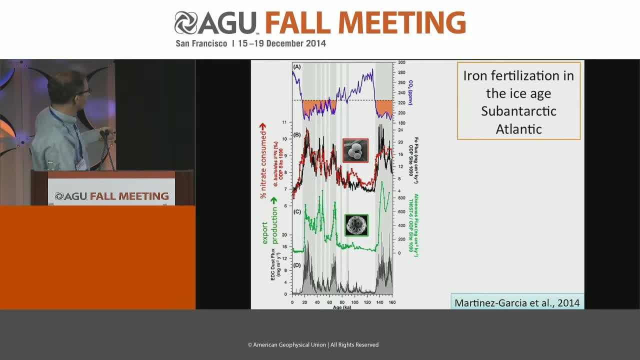 was higher during the glacials in the sub-Antarctic, and you can see that it's even a finer thing than that. This is a reconstruction of export production based on alkanone accumulation rates At each time when dust fluxes are high at the millennial scale, as well as in general. 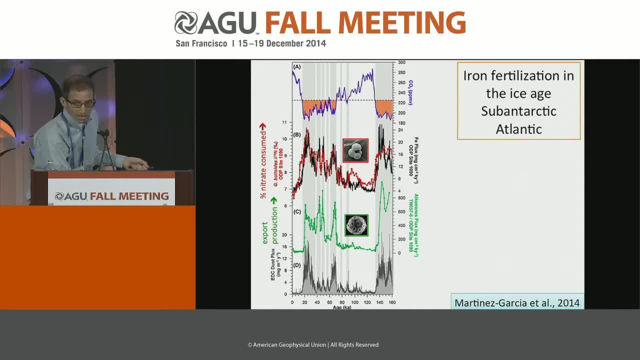 we see higher export production, And so these types of data alone have made people very interested in the possibility of iron fertilization occurring in the sub-Antarctic. However, if that's true, what we should see during each of these rises in export production? 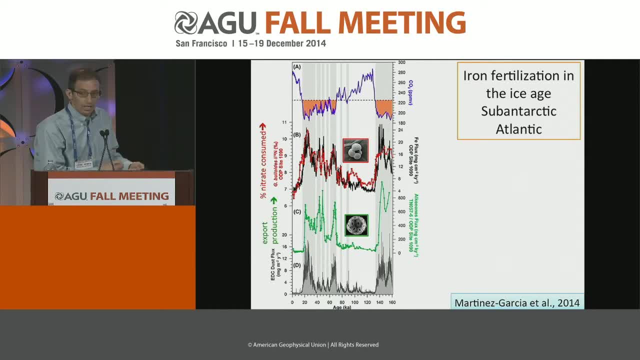 is a decline in surface nitrate concentration, an increase in the degree of nitrate consumption Now shown in the red data. up here are the delta N15 measurements, the red points up here are the delta N15 measurements on the foraminifera gibboloides. 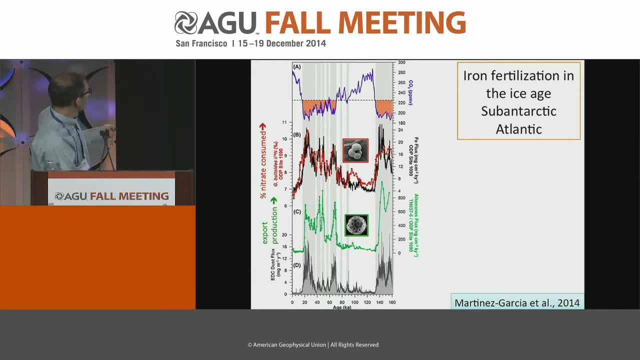 And the red points up here are the delta N15 measurements on the foraminifera gibboloides. And here delta N15 is plotted upward, so higher degree of nitrate consumption would be upward, Higher surface nitrate concentrations would be downward. 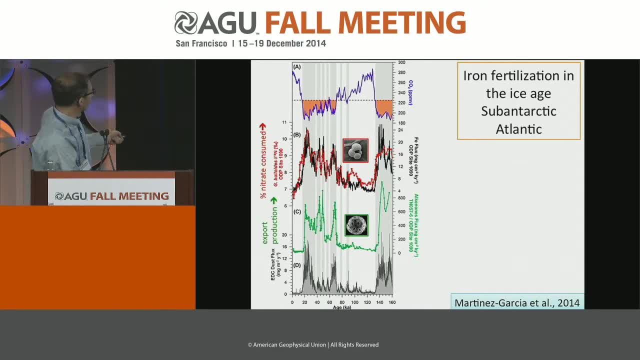 You can see that the correspondence is quite remarkable. whenever there is high dust, there is high production, as we know, and there is also a higher degree of nitrate consumption. It's very hard to explain this data in any other way than iron fertilization. 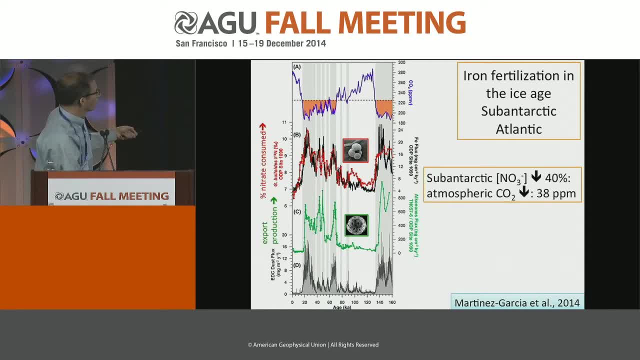 Now the type of CO2 decline we're talking about here, that one would expect from these type of changes, is also on the order of 40 ppm. Some of you might be surprised by that relatively high number, given that the sub-Antarctic ventilates a relatively small volume of the ocean interior. 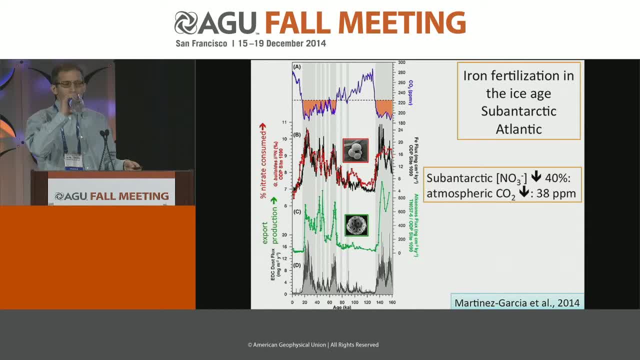 Just hold on to that surprise for a second. The reason you do get such a significant CO2 drawdown is the sub-Antarctic also affects the depth distribution of regenerated carbon in the ocean and it also affects the rate of low-latitude production. 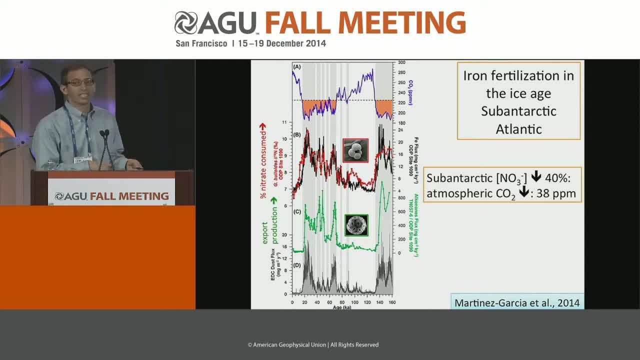 and thus calcium carbonate rained in the seabed across the global ocean, and these things feed back on alkalinity. So the sub-Antarctic takes advantage to a substantial degree of changes in ocean alkalinity to drive part of this CO2 change. 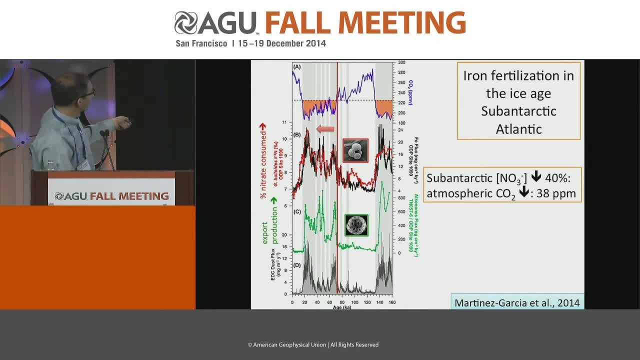 The next point I should make here is that within the last glacial progression, you can see that dust fluxes, and we've known this for a while. don't begin to rise until well into the glacial progression. And, of course, 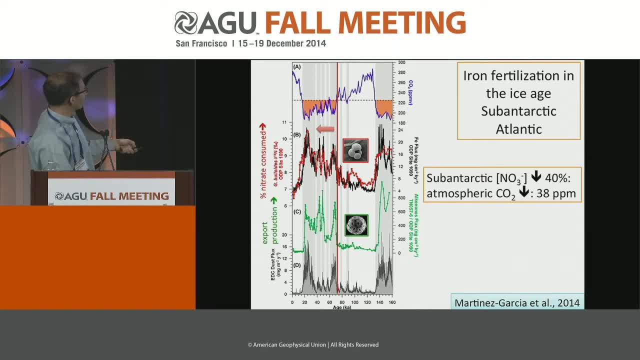 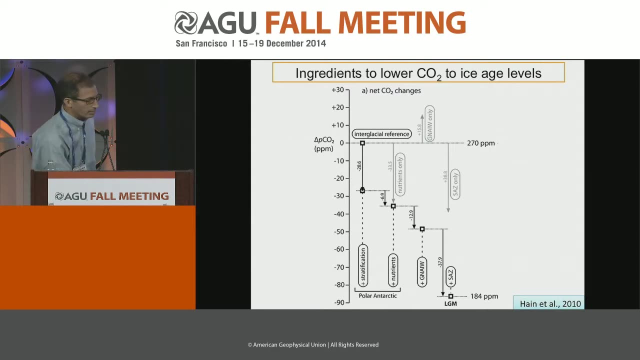 export production, and the first really large changes in Delta-15 occur at that same time. So this iron fertilization seems to be something one might apply to the latter part of the CO2 decline associated with ice ages. So not to be too pedantic about this. 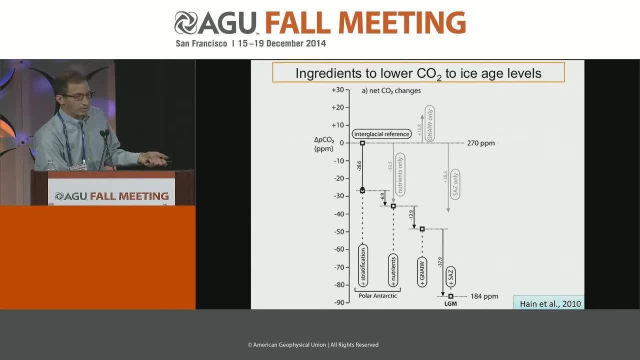 but the argument I'm making here is that Antarctic versus sub-Antarctic changes are both contributing to glacial and interglacial CO2 and the CO2 drawdown over ice ages, but with a different pacing within the glacial progression. 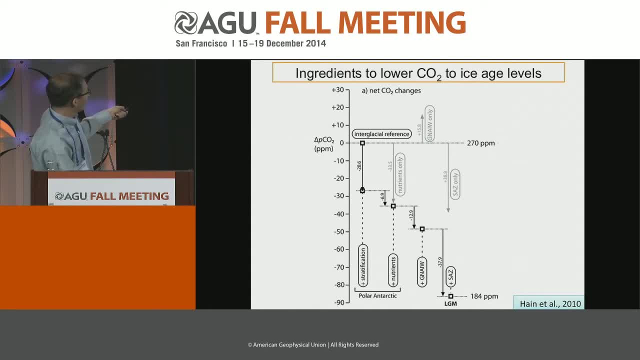 So shown on this axis here- and these are model results- is PCO2 decline going downward here. The Antarctic experiments piled up here in terms of CO2 decline are shown here. So about, in this case shown as 38 ppm, 37 ppm. 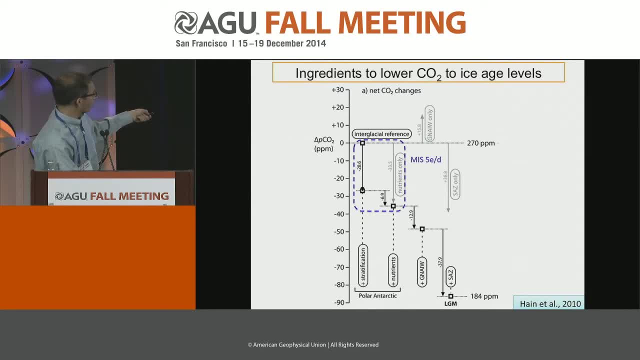 And this, given what I've shown you, one might start to apply right at the MIS-5ED transition, early in the glacial progression. And then these arrows here are for sub-Antarctic zone iron fertilization, as well as the switch from NADW to glacial North Atlantic intermediate water formation. 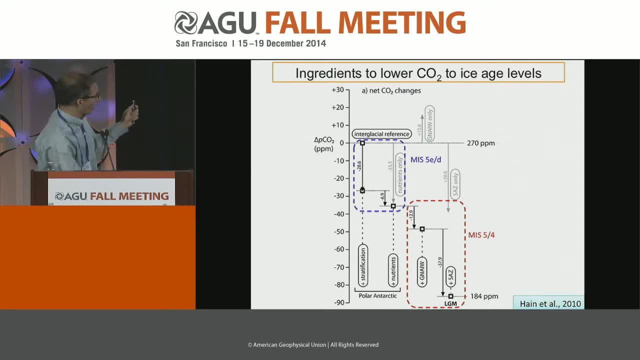 And these, based on the data I've shown you, could be reasonably applied from the 5-4 transition onward, And these together, when you bring them together, can get you to a CO2 drawdown that's greater than 80 ppm. 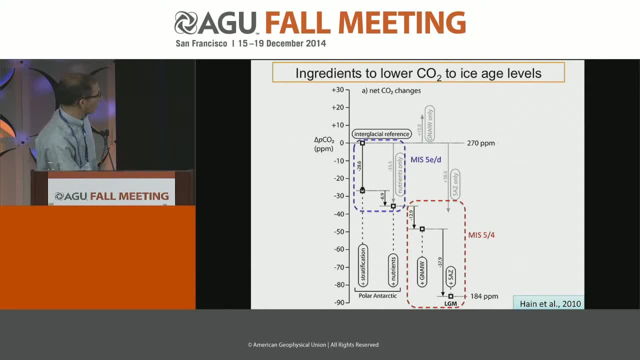 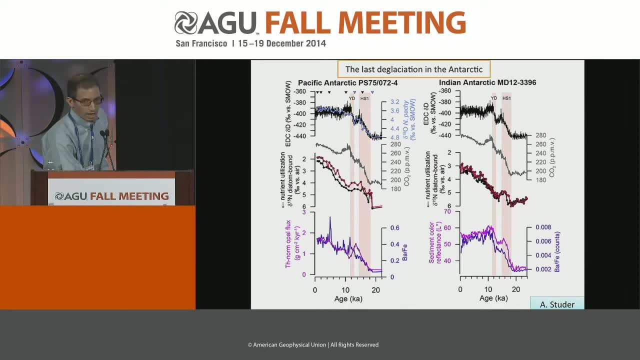 or quite close to the observations for how much CO2 is lowered during ice ages. Now I want to end up by talking about how these things unwind in the deglaciation. We have less information about this right now, but I'm going to show you some of the things we have. 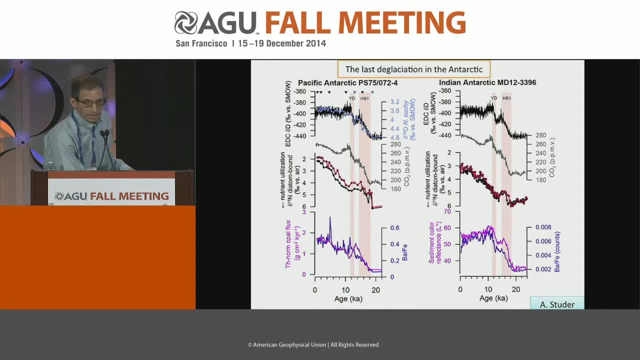 We're going to talk about the deglaciation in Antarctica. So the data on the left here are what I've already shown you but now just blowing up. in the last 22,000 years We have again these same ice court thingies up above. 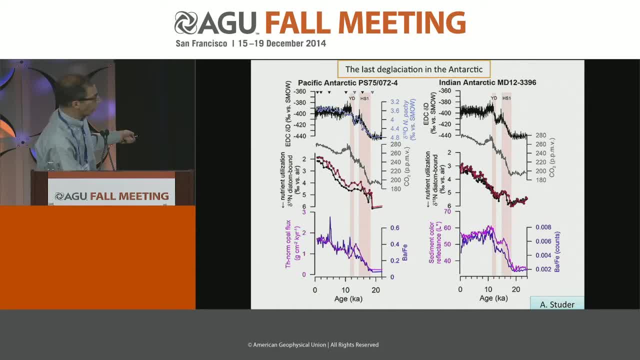 down. here we've got the reconstruction of export production change. and here are the Delta N15 data, again plotted higher, plotted downward. So what we see is, at this time, an increase in export production, an increase- sorry, pardon me, a decrease- in the nitrate consumption. 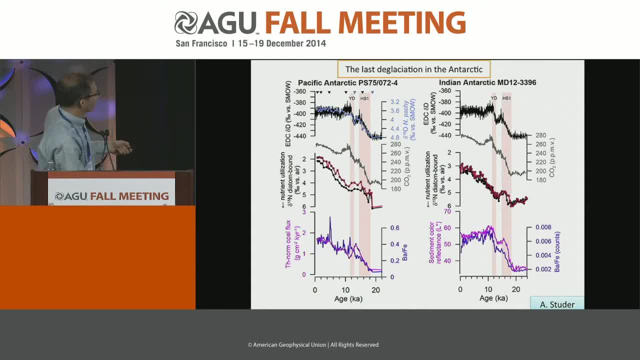 and so it looks like the unwinding of the stratification that applied during the last ice age. Now there's an early part to this, so something that one might imagine applying to part of this is a CO2 rise early in the deglaciation. 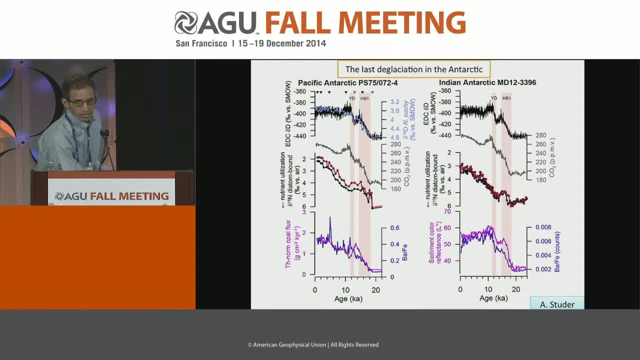 At the same time there's an awful lot of continued Delta N15 fall through the Holocene. Now we were pretty uncertain about this. I could tell you about our tribulations with age models in these Antarctic sediment cores, but we also beyond age models. we were worried about how regionally expansive this signal was. 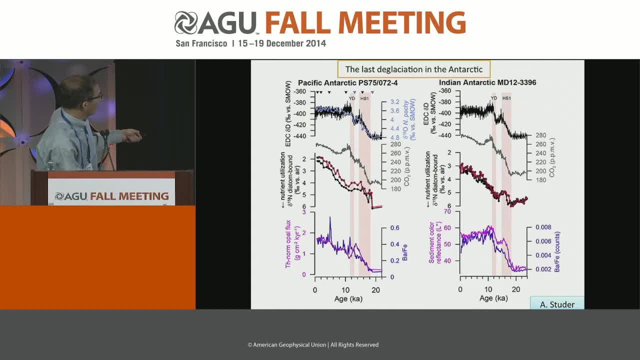 and so we now have some new data from the Indian Antarctic and, without belating it, without belaboring this greatly, these here are the diatom-bound Delta N15 data. They really are there, these red and black over here for the Indian Antarctic core. 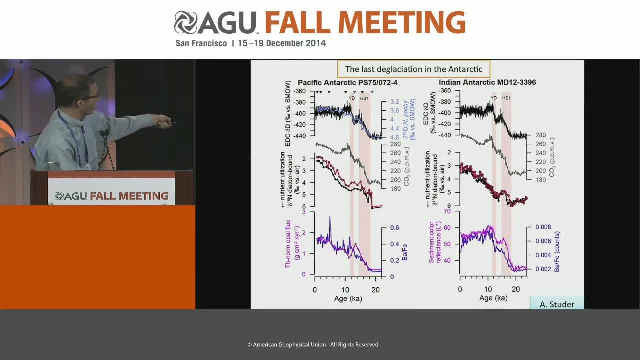 and here are some proxies for export production, similar to the ones that are used over here And again we see an increase in production and a decrease in nitrate consumption, with the first part starting quite early in the deglaciation, at the beginning of what people refer to as HS1,. 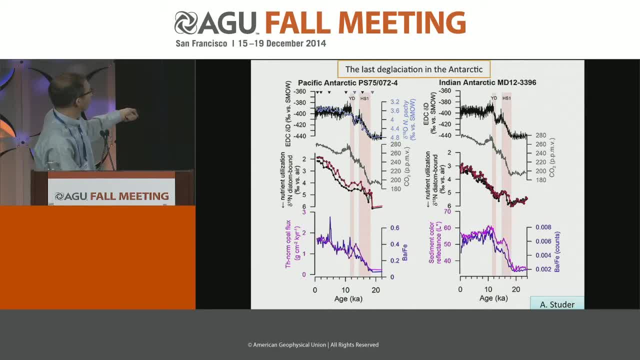 but then much of the further decline in Delta N15 occurring through the Holocene. much is observed in the Pacific Antarctic, so we're starting to believe this Holocene trend. Now this offers both possibilities and questions, and the kind of possibility it raises is that this CO2 rise that has been mysterious. 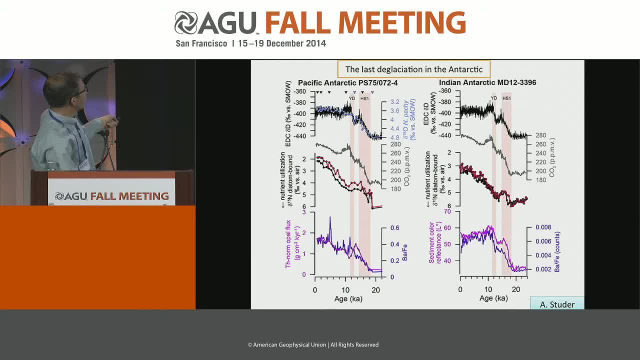 occurring through the course of the Holocene might be explained by this continued Antarctic destratification over the course of the Holocene, something we didn't expect to see. At the same time, it means that you can't imagine that this destratification applied all to the HS1 interval. 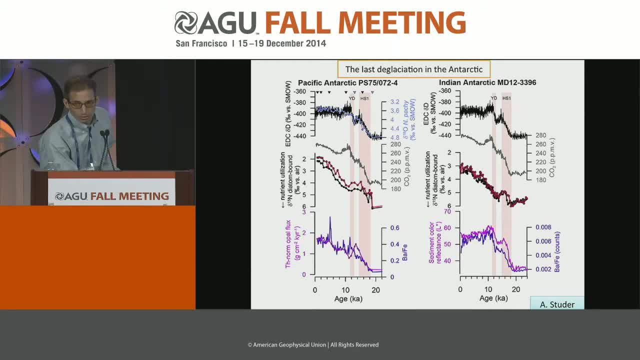 And so some of this CO2 rise is going to have to have other origins, And I don't have the time to defend this now, but the data that we have for the sub-Antarctic would suggest that this change did unwind quite early in the deglaciation. 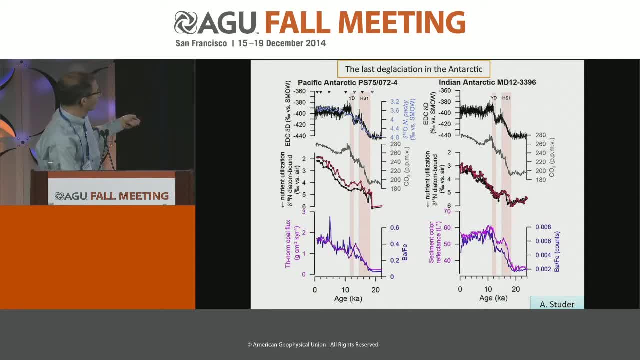 and so we do believe that a lot of the loss of iron fertilization would have applied to the early CO2 decline. And there's also deep ocean warming that's occurring over this time period, and we've just heard something very relevant from Andreas on this matter as well. 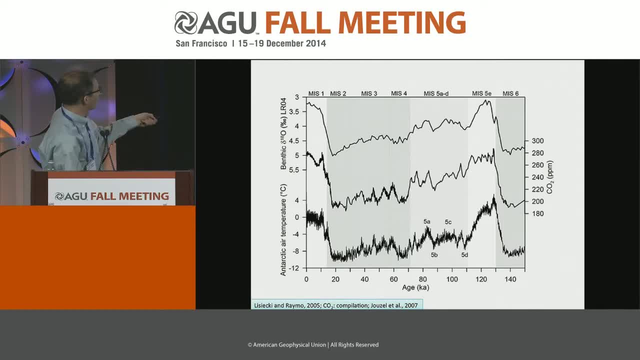 Okay, so to summarize, I have the atmospheric CO2 record for the last glacial cycle in the middle, which is flanked by the oxygen isotope record and Antarctic air temperature from Antarctic air temperature, and so we have the interglacials here and here. 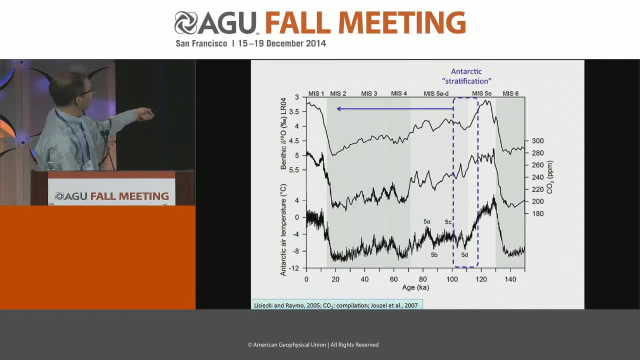 And so what I'm proposing is that, starting at the end of the previous interglacial, the 5-ED transition Antarctic stratification began to apply itself. That drove some of the early CO2 declines, and this continued through the full glacial to the last glacial maximum. 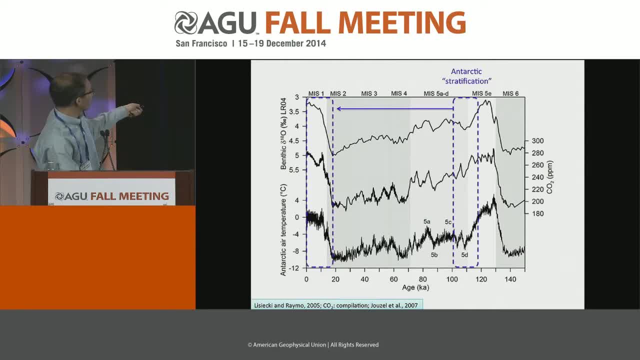 And then it unwound, starting in the beginning of the deglaciation but also continuing through the Holocene. Sub-Antarctic iron fertilization appears to have begun about halfway through the glacial progression and may explain this latter part of the CO2 decline. 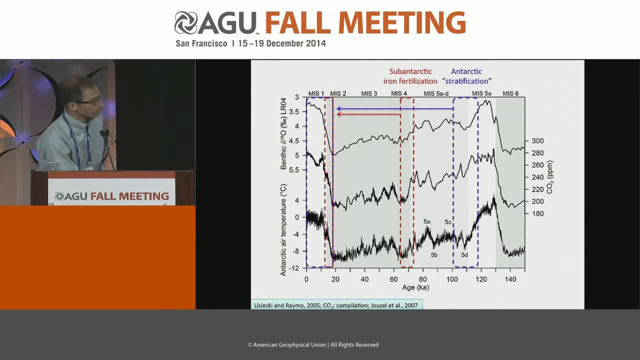 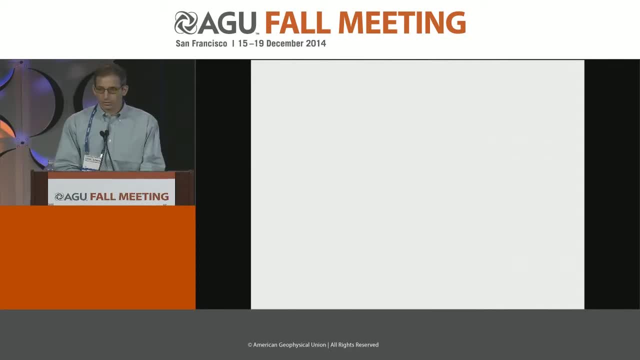 and it appears to have unwound quite early in the deglaciation. That's it, Thank you. Quick question and then we have the other group coming in. Anyone, Ed Danny, one of the ice core observations is that some of the CO2 changes during the deglaciation are very fast. 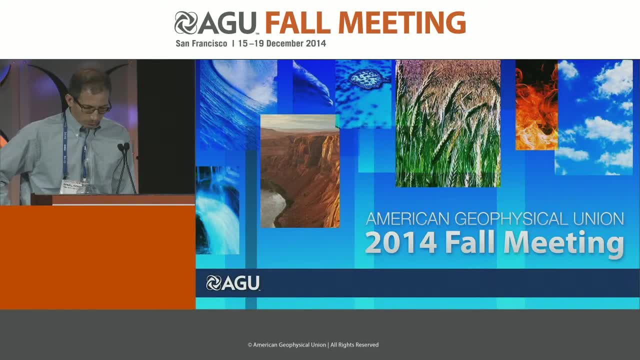 So are there limits? do you think on how fast the mechanisms you're talking about can happen? Yes, Yeah, so a couple of comments. Let me say that Sean, in his email about this session, mentioned these rapid changes, and my talk ended up ignoring them. 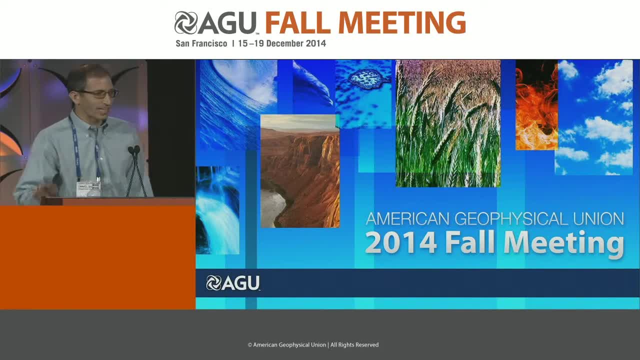 And that's because I thought I would run out of time actually. So we do have something to say about these fast transitions in the deglacial, but it'll be maybe some other time. That said, the deep ocean overturning changes. you know, they have a very fat, they can have a. 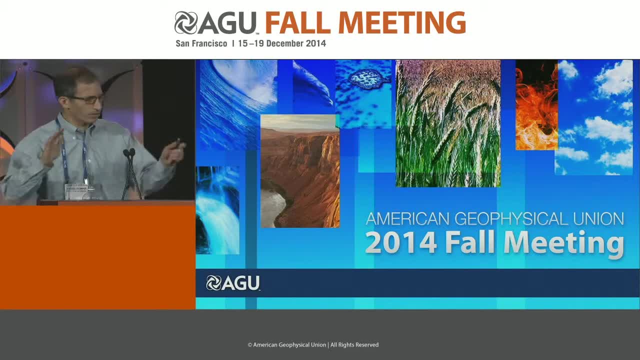 they have a long component, which is the calcium carbonate component, which is thousands of years and isn't relevant to your question, And they have a fast component which involves the venting of respired CO2.. And so does you know sea ice retraction.